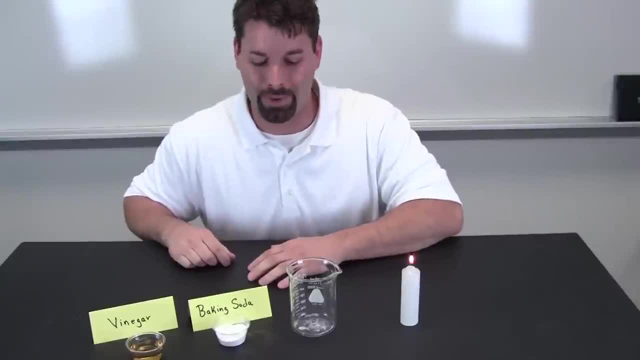 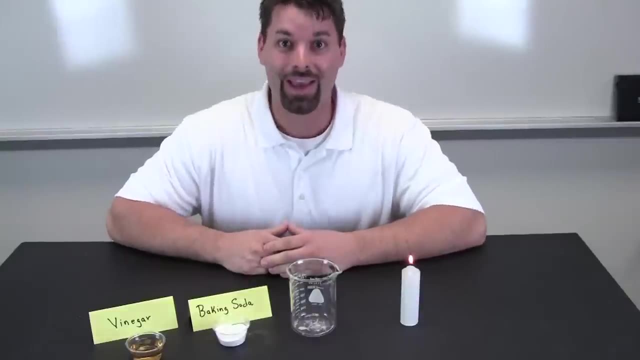 So I have two substances, two materials to make that happen. We have baking soda and we have vinegar. These two ingredients will create another gas. You cannot smell it through the video camera, but you will be able to see it A la the candle. 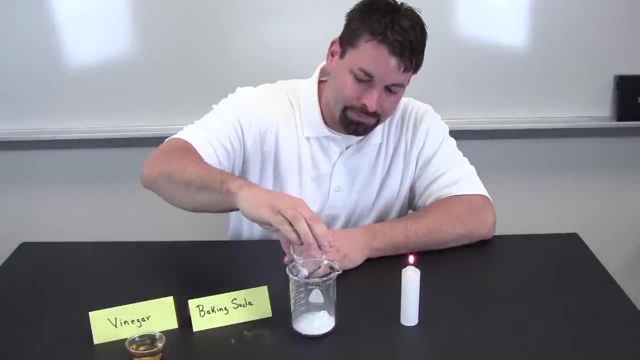 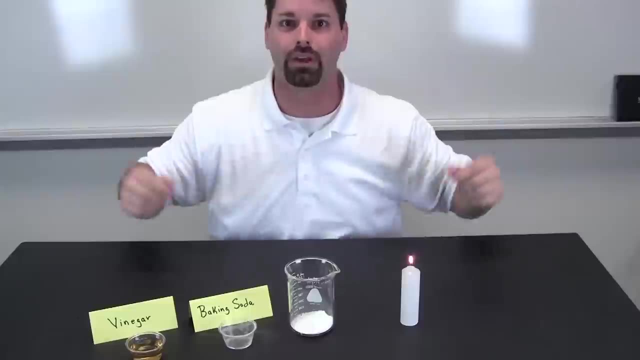 So here we go, We are going to dump in the baking soda And when I add the vinegar, I should get a reaction. How do I tell it is a reaction? It is going to bubble, It is going to foam. It is not going to pop up like a volcano, but you are going to see the fizz happen, almost like soda. 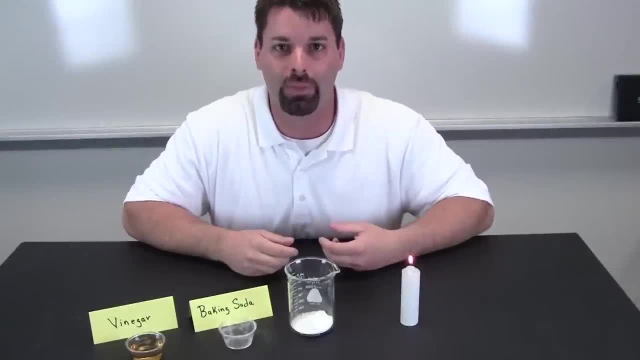 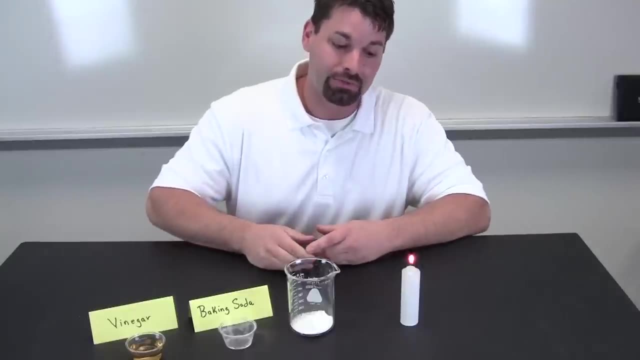 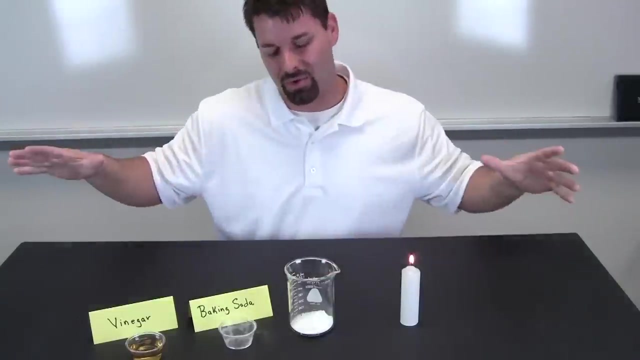 A gas has given off. What do you think is coming out of those bubbles? Well, it is actually carbon dioxide. Carbon dioxide is not oxygen. Carbon dioxide should be able to extinguish and put out this flame. It is actually a lot heavier than the air around us, so it should stay in the beaker. 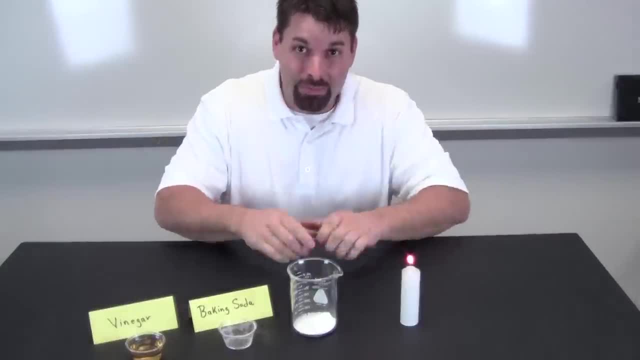 It is not going to be spilling over the sides. You could not see it. It will stay in the beaker and I am going to prove it to you. Now for the science, We add the vinegar. Now for the science, we add the vinegar. 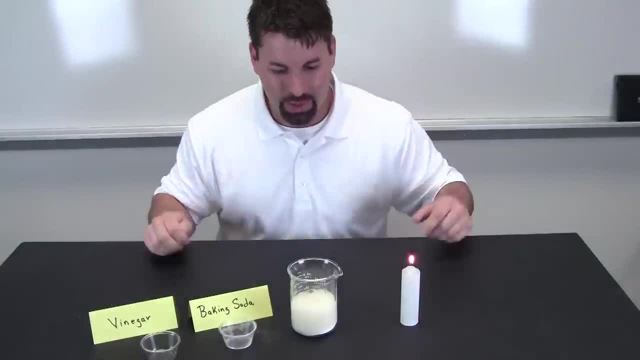 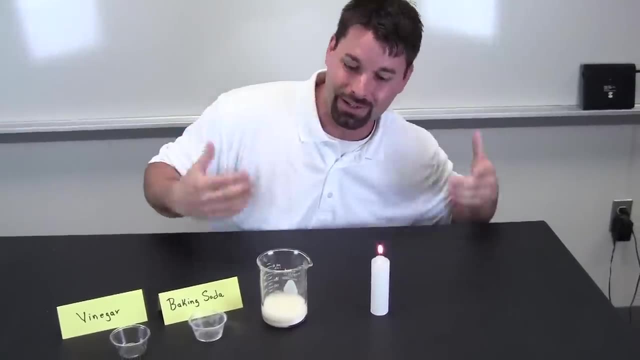 You can see the reaction, The foaming action, the bubbling, the popping, Plop, plop, fizz, fizz. Oh, what a relief it is. There is gases being released into that beaker, but you cannot see it, and neither can I. 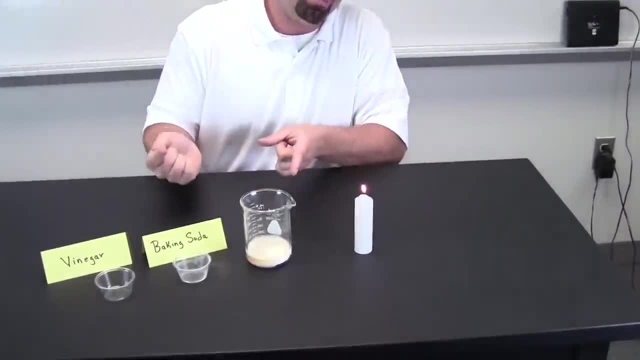 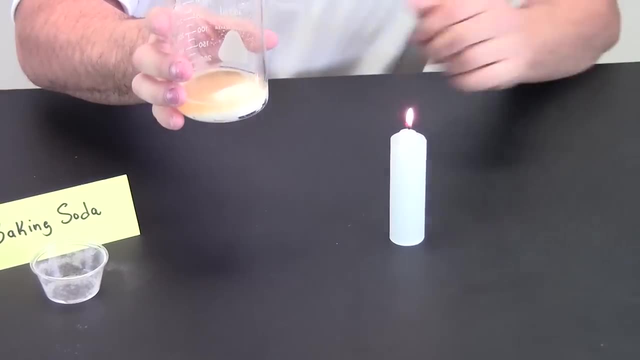 It is in there. It is heavy, So I should be able to actually pour the gas onto the flame and watch the flame go out. This is the cool part. I am not going to pour any of the liquid. I am going to pour the gas out of here onto the flame. 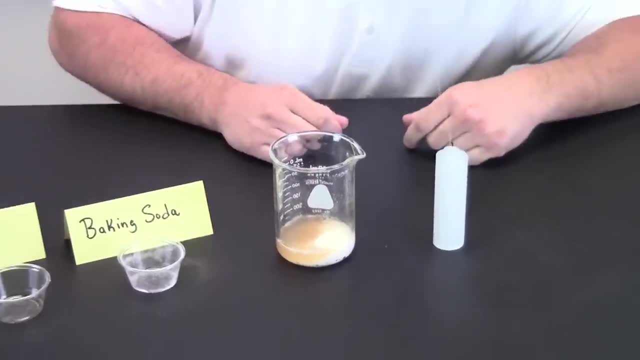 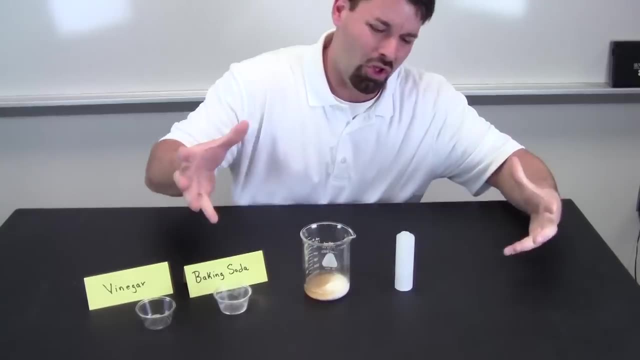 Whoa, I did not blow that candle out. The carbon dioxide smothered it. It is kind of like putting an invisible blanket on the flame. Oxygen cannot get to it. All the carbon dioxide swirls around that flame. The candle cannot take any of the oxygen in the air. 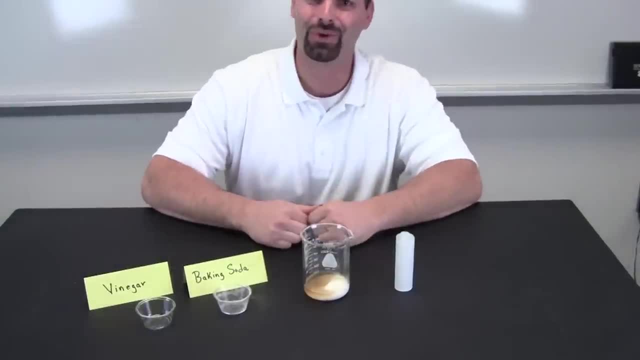 The carbon dioxide put out the flame. Science is so cool. Thanks for watching.